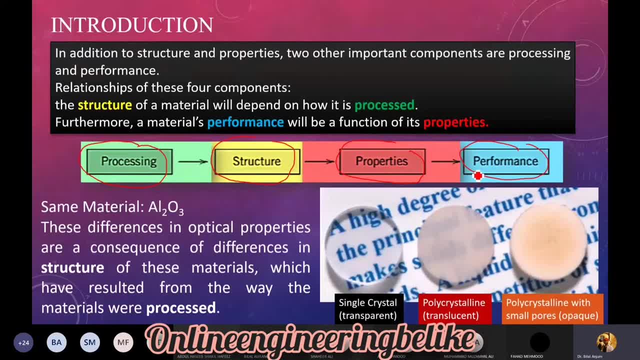 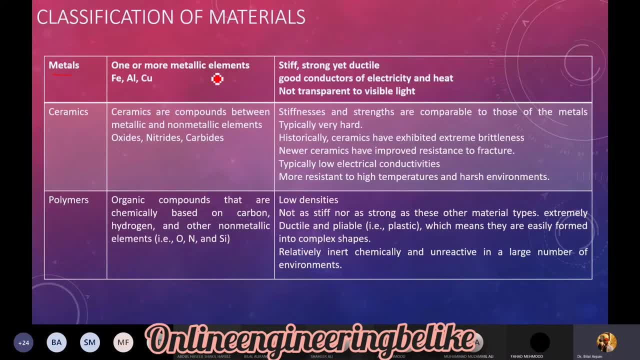 categories of materials that exist. The first one is metals And, as the name says itself, it is made up of one or more metallic elements. the material- iron, aluminum, copper, steel- is an alloy of two components, which is iron and carbon, still a metal, The generic. 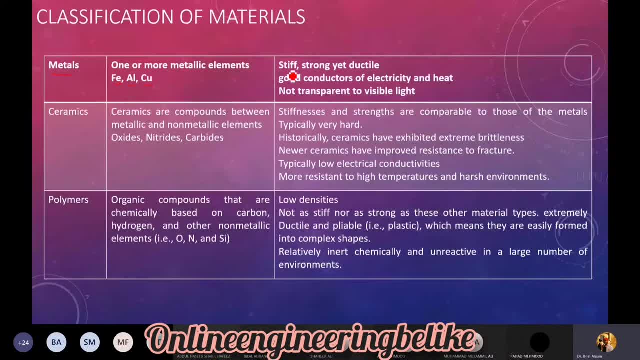 characteristics of metals include stiffness- they are strong, yet they have good ductility. they have got good conduction for electricity as well as heat, and they're not transparent to visible light. General characteristics of materials belonging to the category of metal. Then comes the important category of ceramics. 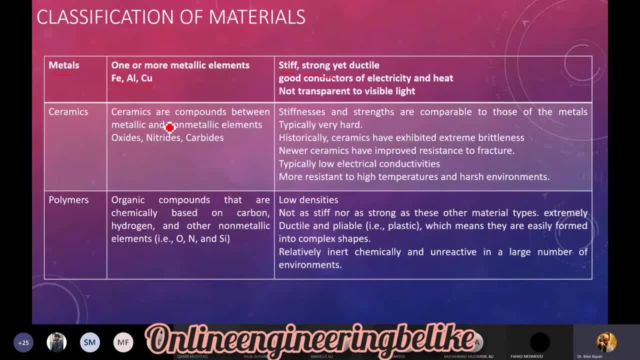 ceramics. they are compounds between metallic and non-metallic elements, and they are commonly oxides, nitrides or carbides. These are normally characterized as ceramics, For example, the material that we learned about in our earlier class, alumina or Al2O3,. it's a ceramic. 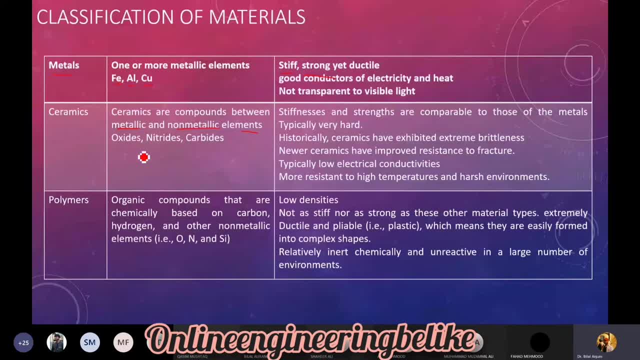 Similarly silicon oxide, silicon nitride. they are compounds between metallic and non-metallic elements. They are also ceramics. General characteristics: they have very good stiffness and strength and their strength and stiffness are comparable to that of metals and they are very hard. Stoically they have been known for their 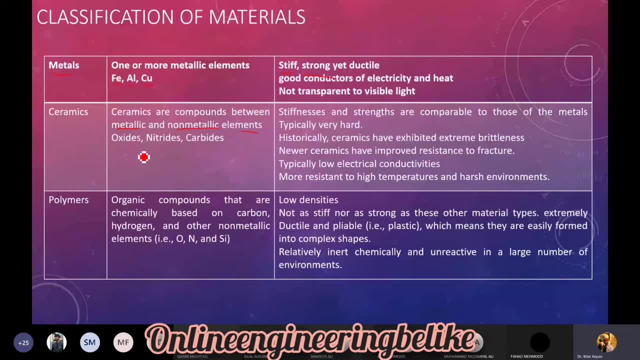 brittleness that they are very brittle in nature. they are not as ductile as the metals. However, the new ceramics are now very fine, but they will get very damaged. Still their they have improved the fracture resistance or the resistance to their brittleness. It has improved 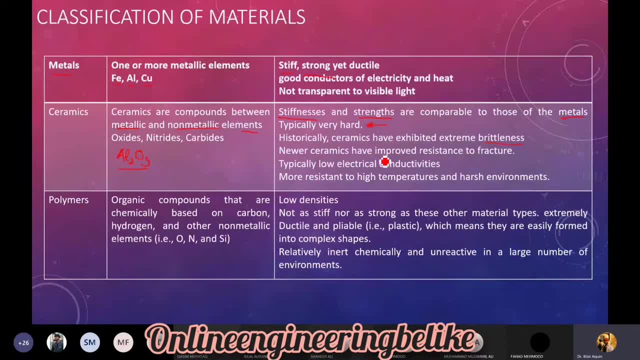 to an extent, but still they are categorized as brittle as compared to metals. Again, typically they have low electrical conductivities and they are more resistant to high temperatures and harsh environments. So ceramics mostly. they are used for applications which require high temperatures, For example your furnaces. they have the insulation made up of alumina. 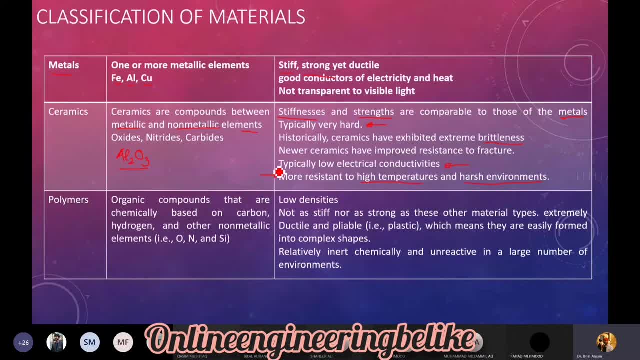 which is a ceramic, So high temperature applications or applications that require resistance to harsh environments, Ceramics are normally used in those environments. The third category is polymers. I'll write your name in the chat section. I'll not mark it, So don't waste your time. The third category: 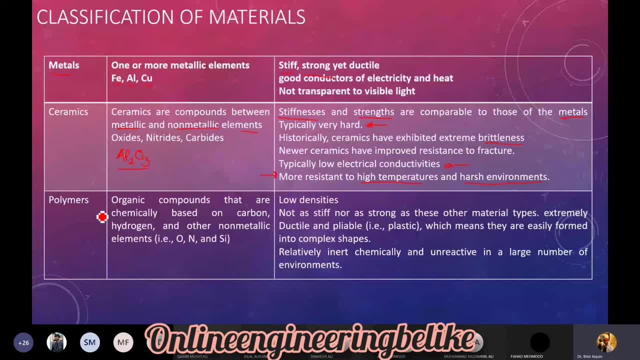 is that of polymers, and polymers are made up of organic compounds that are chemically based on carbon and hydrogen and some other non-metallic compounds. So polymers are made car tz more. No, It's more about the. They are, it's western. that. that's what makes polymers more. the environment stats What makes polymers more difficult. Let me tell you aboutbilir Too much have recorded could be found to yourself. It can make anyone wonder how these pictures happen to me far. 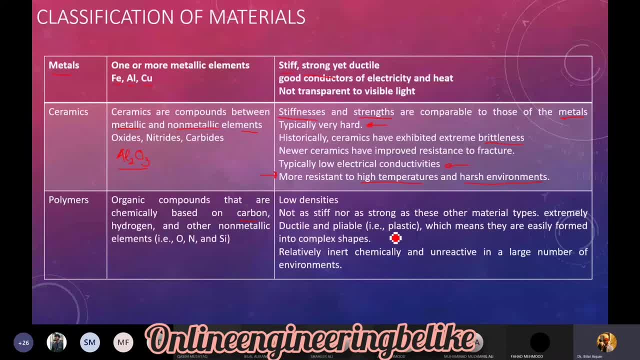 We should talk to make this possible. John, Tony, giving us a buzzard more useful these days. these are the three broad categories of materials that that you should have the basic understanding of our. our focus mostly would remain around the metallic systems, although we'll have a discussion on ceramics for even composite at the end, but primarily we will focus. 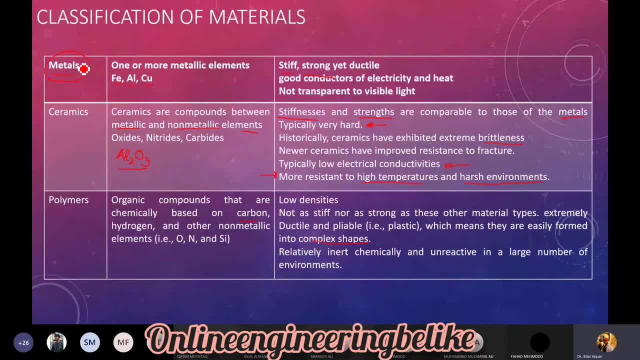 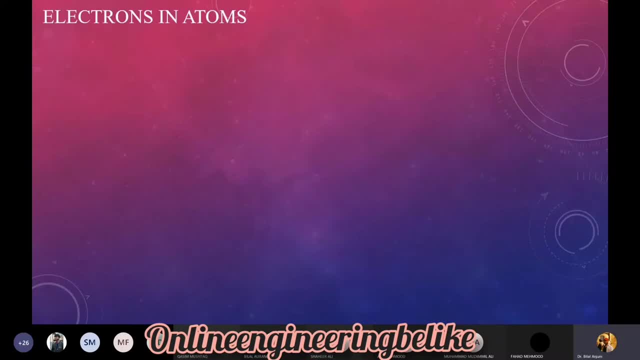 on metals as they're mostly used: uh. now, moving on towards some of the big basics of high school that you must be familiar with: uh: electrons in atoms, the, the convene, the original or the traditional simplified bohor atomic model. uh represented that electron are assumed to revolve around the atomic nucleus in heat orbitals. 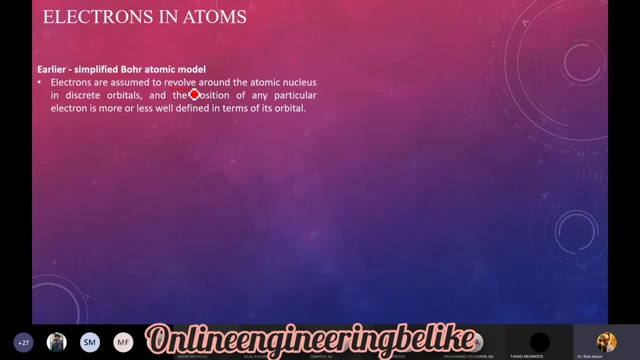 and the position of any particular electron is more or less well defined in terms of its orbital, also discrete, that means the energy states do not vary continuously with energy and there are finite energy steps that that are there within the electronic structure. for instance, if you look at this uh original model. 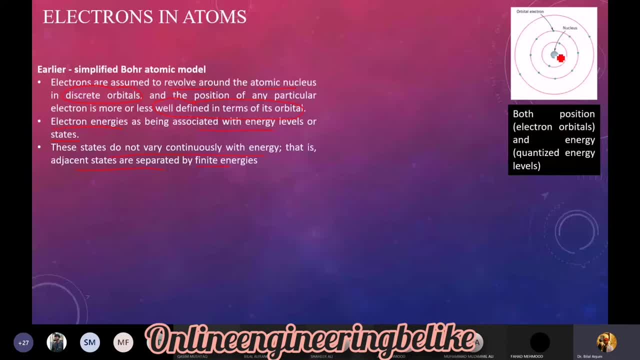 you have a nucleus over here and at a certain distance from the nucleus you have the first orbital that would contain the uh electrons and similarly the second orbital and third orbital, and this orbital would have a finite energy as compared to this orbital and this orbital, but there would not be any energy levels in between, so there would be discrete energy levels and 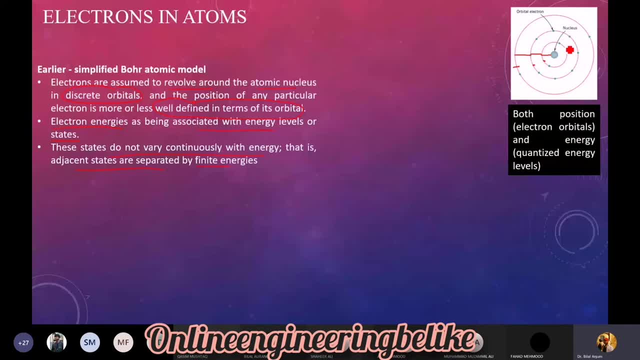 electrons would be quantized at different energy levels. uh. this was the original uh or simplified bohor atomic model, but later on the the wave mechanical model, it. it indicated that electron is both the wave-like nature and the characteristics. that means electron is having this movement of wave-like nature present within itself, along with the particle nature. 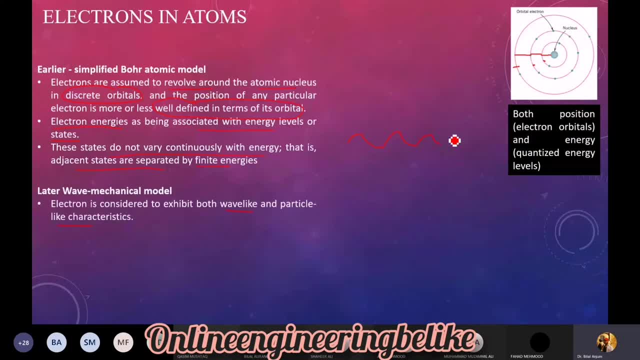 this means that can be moving in a discrete orbital, that the, the orbit or the electron moving within this orbital motion. uh is only a portion of it, which is correct also means that electronfund is essentially moving in a wave-like, so this electron motion is actually depicting both the particle-like nature and the 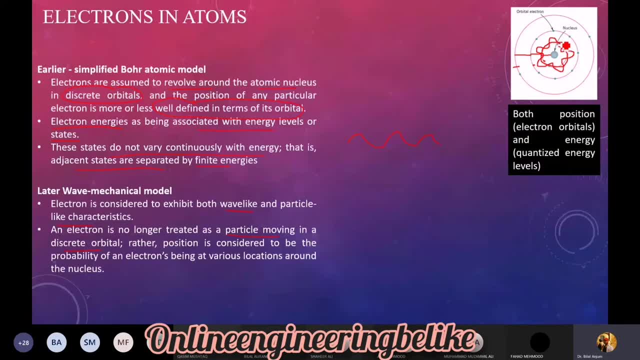 wave-like nature, and this makes the fact that stemmed from this wave-like nature, In other words, position is then described by the probability distribution or electron level. How do you? Yes, sir, Is it better now? Yes sir, Yes sir.